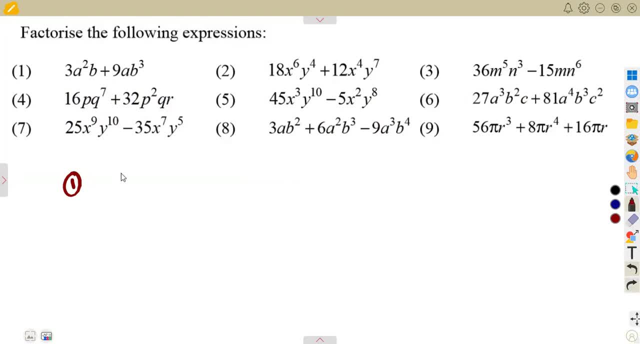 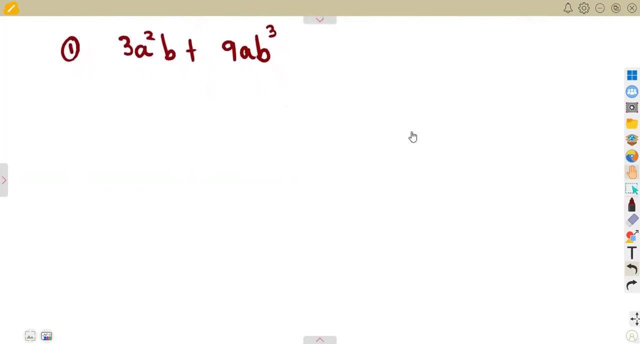 same thing, so there's nothing new there. Number one: we are given 3a squared b plus 9ab to the exponent of 3.. Okay, that is, you are asked to factorize this. Remember I said: every time: consider the highest common factor. check, Are we having? 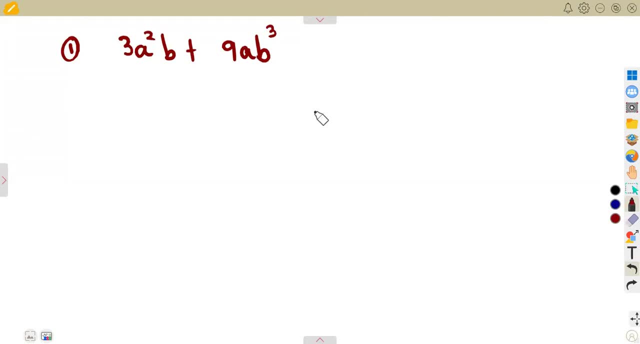 that Talk of the numbers. there's a three and there's a nine. What is the highest common factor between three and nine? Three is already a prime number, So there's no way we can have another number bigger than that. So meaning to say three is the highest common factor between three and. 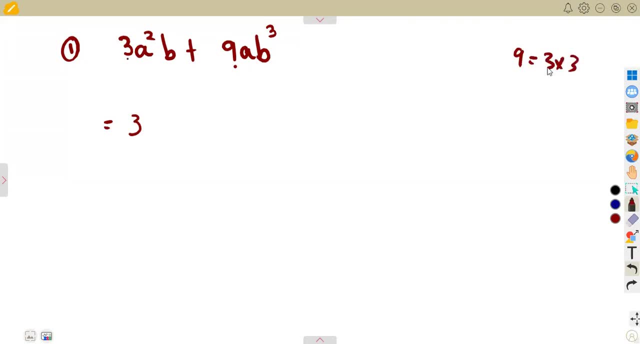 nine. Remember, nine is a product of three and three. So meaning to say three is common, three and three. So you're going to take three. Then, in terms of the letters, I explained that whenever you're given variables, the first thing it is: supposed to be common. like what a is what? like what is happening on a? a is common, We have got a, we have got a, but this is a to the exponent of two, this is a to the exponent of a one, So you, 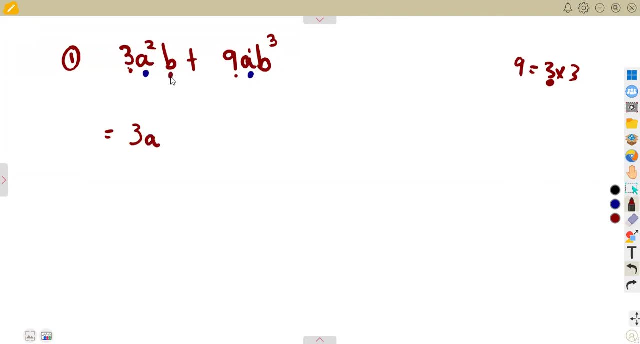 factor, the one with the smallest exponent. There is a b. there is a b to the exponent of. three is common between the two terms, But which one is for the smallest exponent? That is a b. So that is your highest common factor. The highest common factor is supposed. 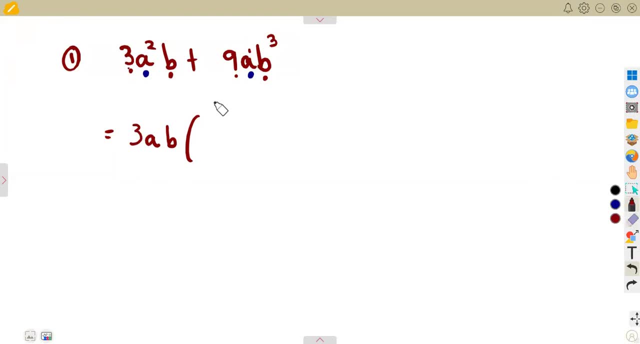 to be having the smallest exponent in terms of the variables with your highest common factor that you figured out. you have to divide these to the highest common factor. I explained this: three a squared b. when divided to three a b. what's going to happen? this and this will cancel. 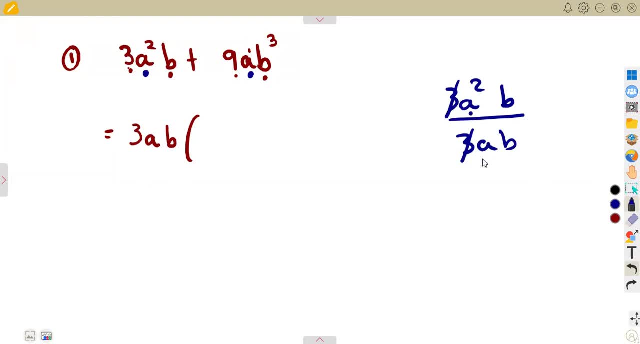 There are two a's here. Here there's only one a. so this one a into these ones, we are going to have one. we are going to remain with only a single a. the b and the b will cancel each other, So that means we are just left with a there. 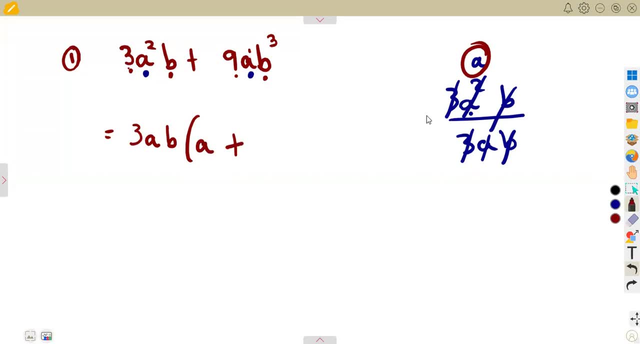 So that is the idea. Plus, we divide again with the same concept. but I say, remember I said on the introduction supposed to do this in your mind: nine and a three, that is going to give us a three. if you divide the a and the a are the same. 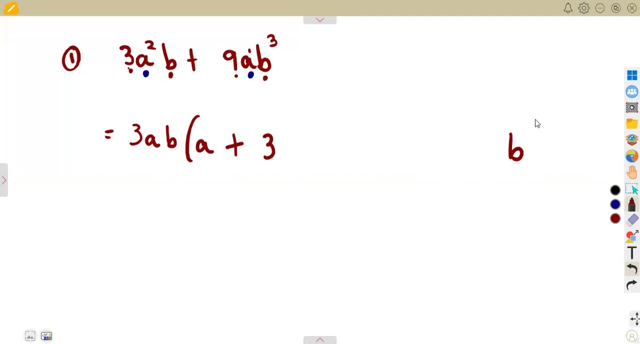 the b to the exponent of three to the b. there are three b's. here you are dividing by a single b, there there are three. So if I cancel I'm just going to remain with two b's. So that will be three b squared. 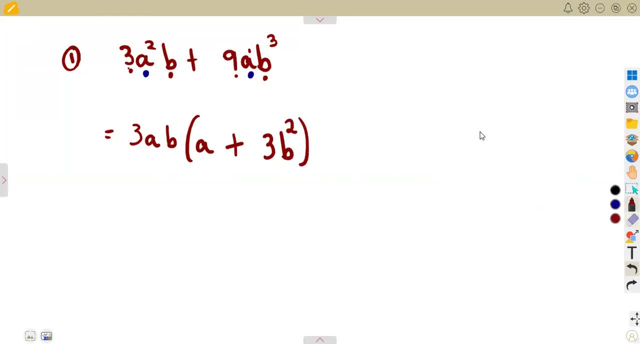 Remember the concept of an exponent means b times b times b. there are three which are being divided by, so this one and this one cancels. you remain with two b's, So it's b times b, which is back to b, to the exponent of two, just like this part. 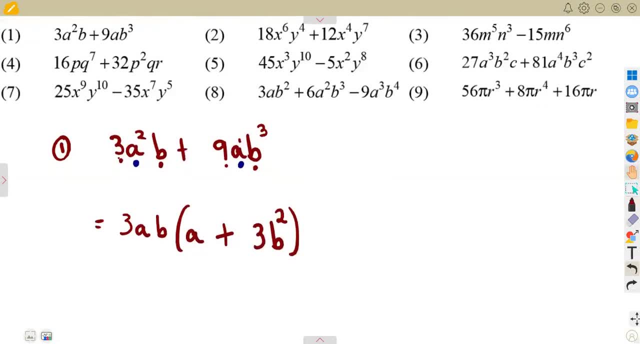 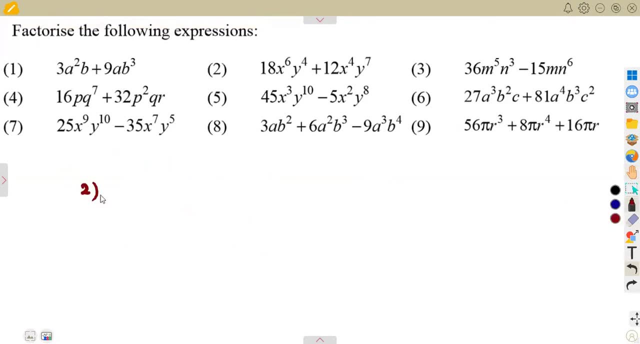 So that is it. That is how you simply factorize this. All right, let's consider number two. As you can see, these ones- they are now easier to answer because we had an introduction about this, So just have to continue answering your questions. Do as many questions as you can. 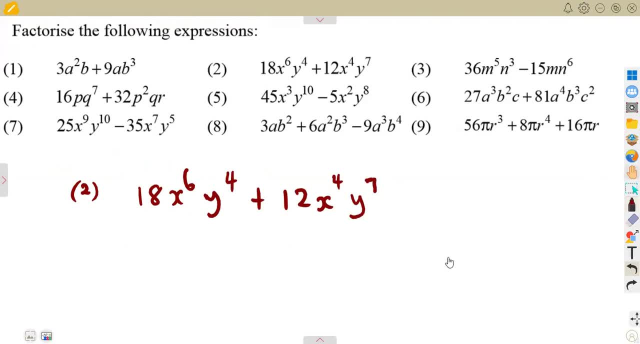 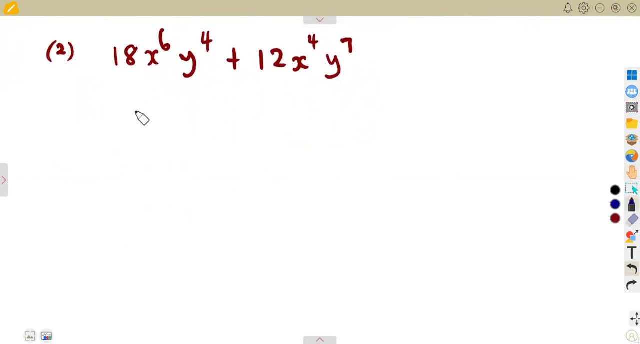 That is the best. Revise as many questions, question papers Also, you'll see that we do not have a challenge. We're not going to have a challenge In mathematics, actually. All right, let us consider these two numbers that we have. 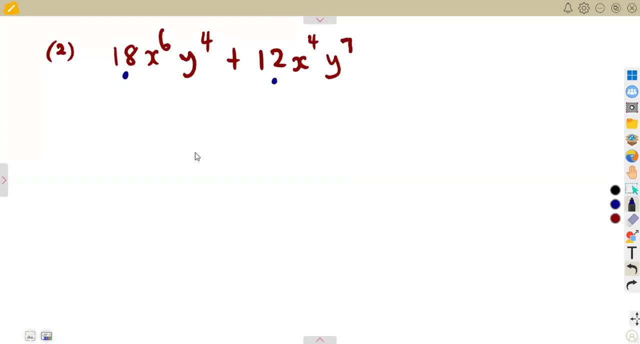 There is 18, there is a 12.. So if I do not know the highest common factor between these two numbers, we are supposed to actually say, okay, there is six, which is the highest common factor, But in a case that you fail to recognize that six is the highest common factor between these two, 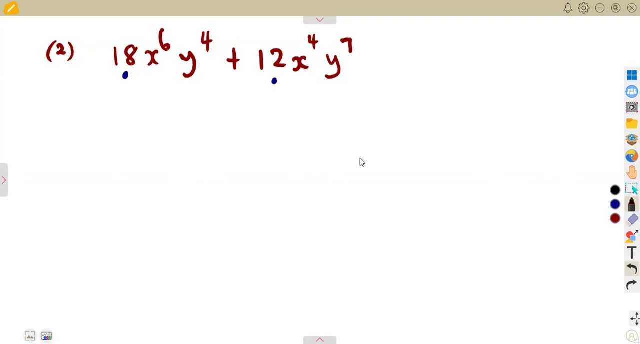 remember I said six is the highest common factor between these two. remember I said, using the manual way of our calculations, we are going to have 18 as a product of its prime factors, The smallest prime factor, which is two. 18 divided by two, that's a nine again. 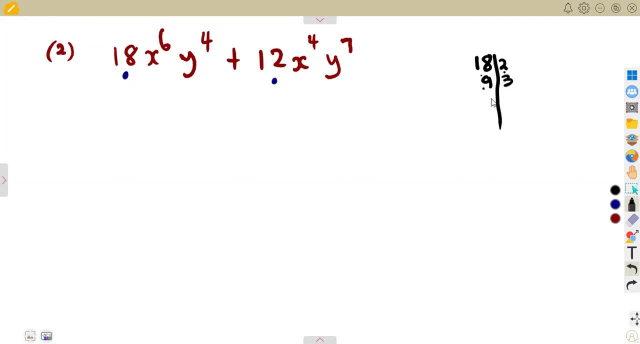 smallest prime number, which is three. nine divided by three, that's going to be a three. again by three. three divided by three, that's a one. All right, we are done with this 18.. We have a 12,. we do the same thing on 12, we divide smallest number. 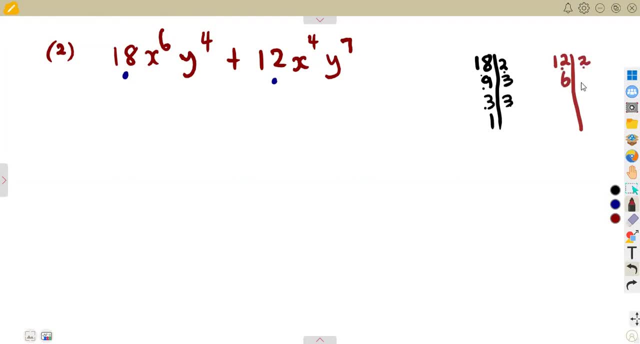 which is two. 12 divided by two, that's going to be a six. again by two. six divided by two, that's a three by three. three divided by three, that's a one. So if we are to consider the numbers, 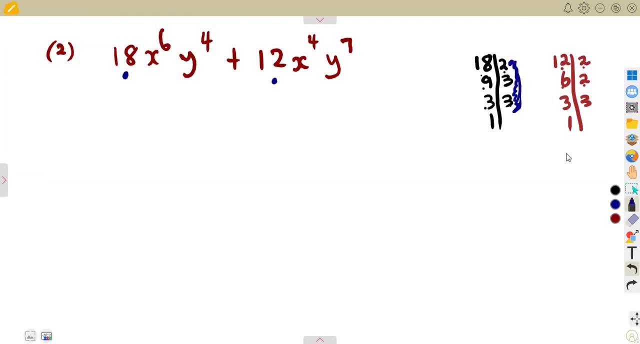 that we are having. these are the numbers that we have, two times three times three. two times two times three. So you'll see that two is actually common between these two, And also there is a three, there is a three there, So it's going to be two times three. 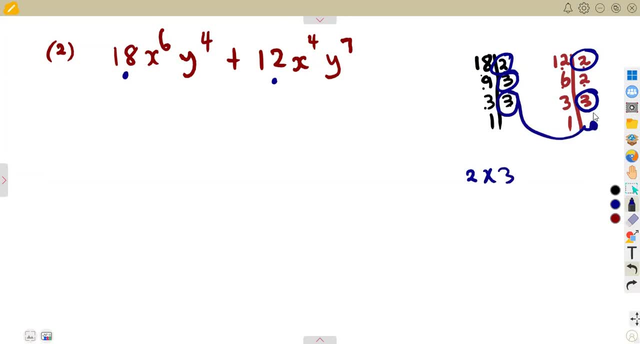 three. these three does not have a number to correspond with. these two does not have any number to correspond with. that is remaining So many to say: we cannot take this, we cannot take this. So two times three was simply going to be the highest common factor. So, like I said, 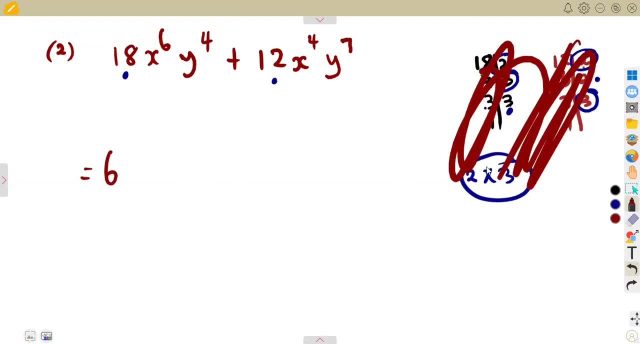 if you know this, there is no need for you to do this. There is no need. but if you are still having a little bit challenge on that part, then I will do the recommend you to use this part. But as time goes on, as you are advised, you see that there. 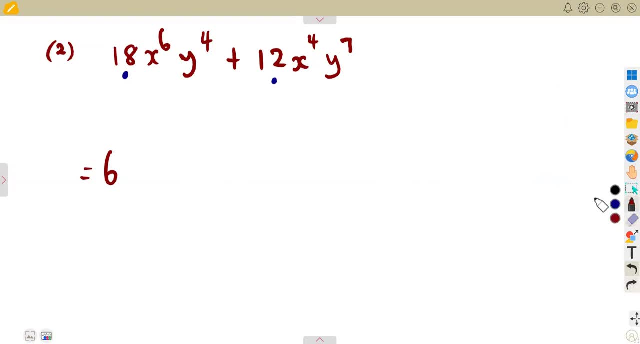 is actually no need is you are doing more questions is okay, there's, you can actually see that. All right, the same way that you're doing on these x here, that there is x to the exponent of six, there's x to the exponent of four, So x to the exponent of four is the one that you're going. 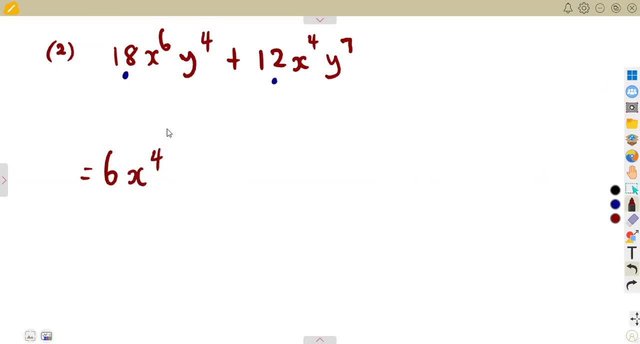 to affect out, as this is the same way that you do even on the numbers when you are now used to them. So do not worry about that. But right, there is y to the exponent of four. y to the exponent of seven. the one with the smallest exponent is y to the exponent of four. 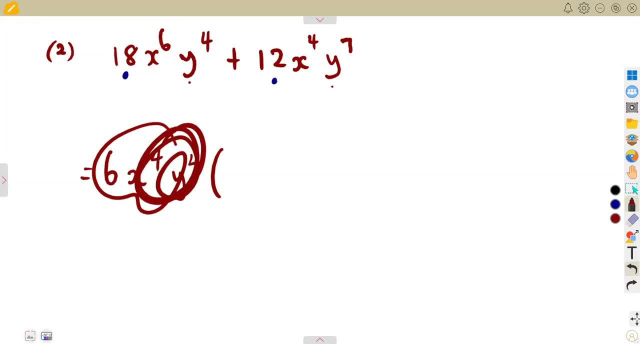 So that is our highest common factor. with the highest common factor we divide back, so that is 18 divided 26.. So, like I say this, if you're also having some challenges, just write it as it is: 18x to the exponent of six, y to the exponent of four, divided by the s2 comma, So divided. 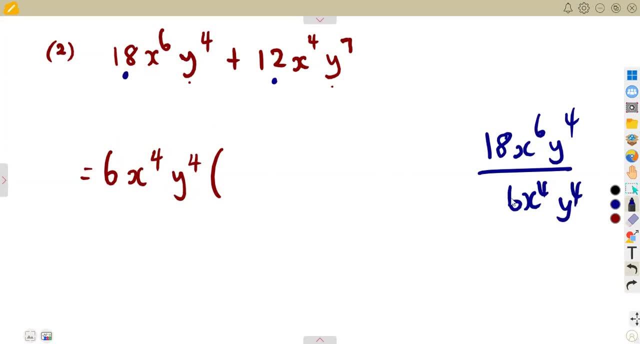 by the st common factor there, what are you going to have at the end? so 18 divided by 6, or 6 into 18, that is going to be a 3, okay, and x. here there are 4, here there are 6. so if we cancel these 4, 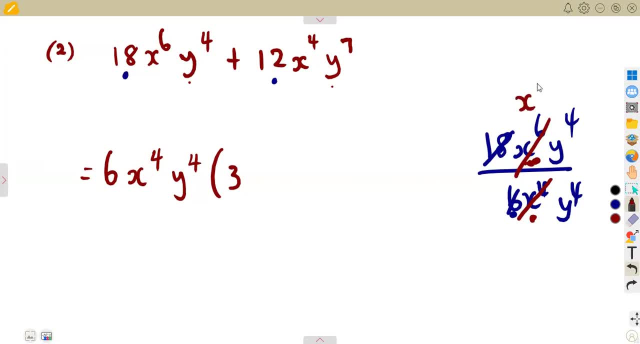 to the 4 that are here, we are going to remain with only 2, so that will be x squared, or you simply subtract the exponent, since you're dividing the bases, which are the same. so it's going to be 6 minus 4, which is a 2. the y to the x point of 4, the y to the x point of 4 are the same, so they. 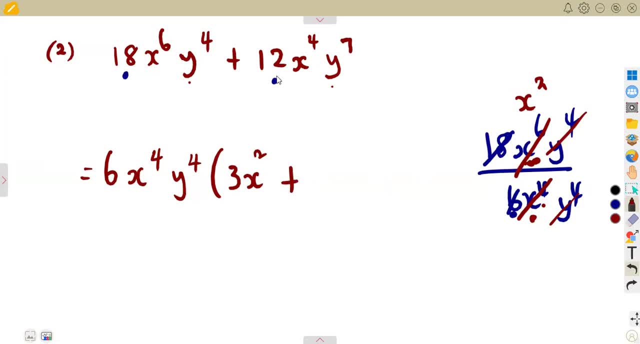 will just cancel. so that's it. plus, you do the same thing, uh, on this part of uh, 12. so there is 12. x to the x point of 4. y to the x point of 7, everything over 6. x to the x point of 4. y to the. 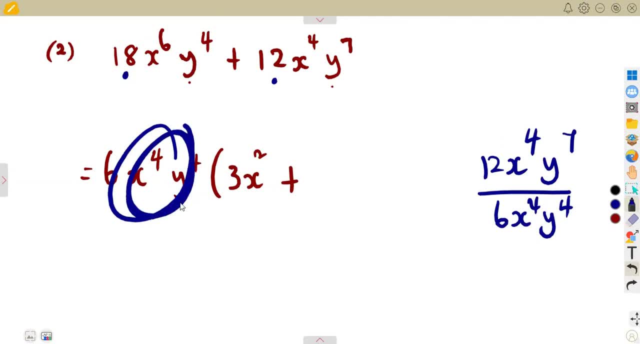 exponent of a 4, which is your highest common factor. so this: if you were to divide the- uh, the 12 divided by 6, that's going to be a 2. okay, these are actually the same for these y's that we have. there are 4 here. yeah, there are 7. so if we just cancel 4 here, on these ones, which 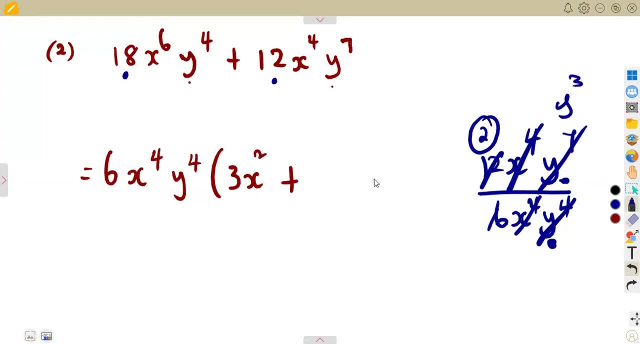 are 7, how many will remain? only 3 will remain. so, oh, just subtract 7 minus 4, that's a 3. so that will be the idea there. 2y to the x point of 3. so that's it. that's the idea of the factorization. 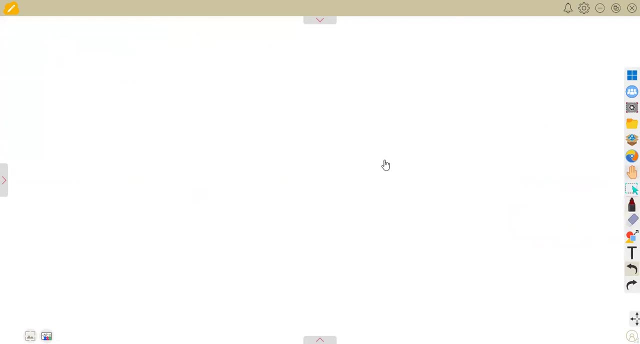 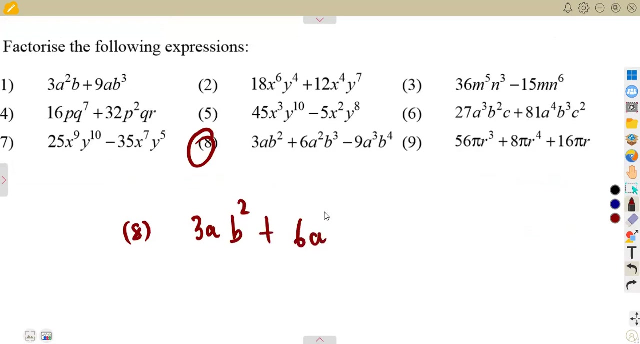 factorization. be careful on how you factorize uh the questions. so they can also be three terms, like what we are given on number 8. we are given uh 3ab on number 8, that is 3ab squared plus uh 6a squared. b to the x point of 3 minus 9. a to the x point of 3. a, b to the exponent of a, 4, so given: 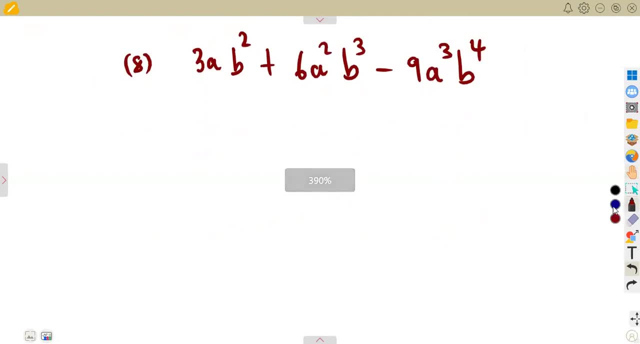 this situation that we have here. we consider the numbers throughout must be common. everything must be common. so 3, there is a 6, there is a 9. what is the highest common factor? by just looking into these numbers, guys, we'll see that 3 is the highest common factor. let's move on to the letters. there is letter a. there is also a to the. 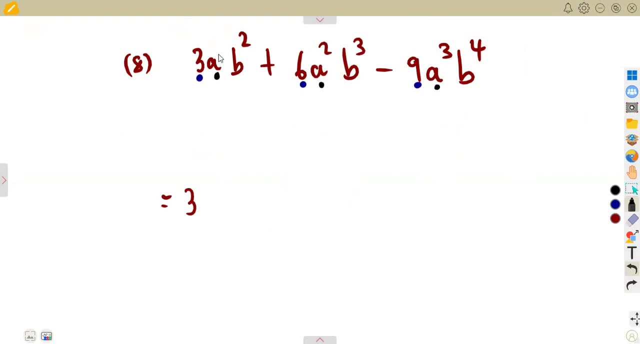 exponent is a there, which one is called the smallest exponent, that is, this one of a to the exponent of one which is just a. considering the part of b, there is a, b squared, b to the x point of 3, b to the exponent of 4, which one is for the smallest exponent, b to the exponent of a, 2. so 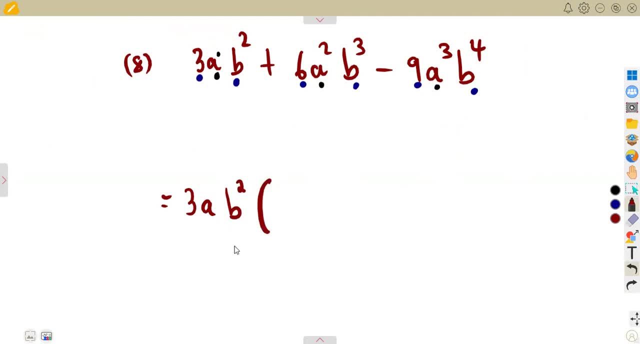 this is your highest common factor. with the highest common factor, you divide each term back to the highest common factor. so, in actual sense, you were supposed to divide these, uh, three, a, b, squared, divided to this, but, as you can see, they are actually the same. so the three and the three. 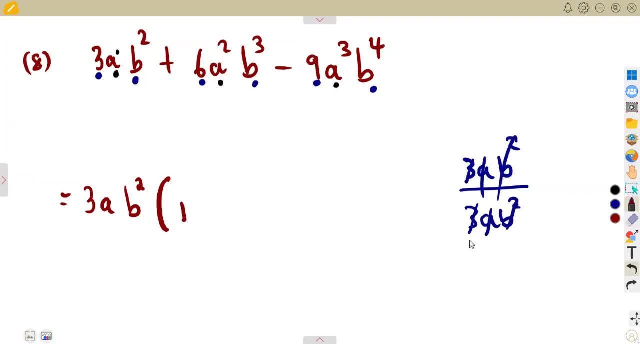 so the a and a guys, this is just a one day. okay, we move on to the other part. there there is a 6a, so this will be plus. there is a 6a squared b to the exponent of three, everything over three. a b to the. 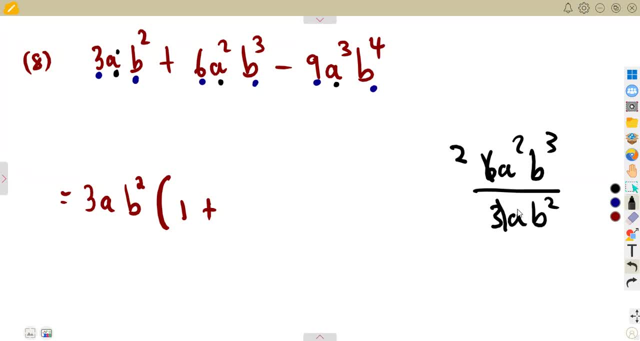 exponent of two. six divided by three, that's gonna be a two. a into these a's which are two, that's gonna remain with one. or just subtract two minus one exponent. the bases are the same, just like this: the base of the same subtract, the exponent. so three minus two, that will be a one. so meaning so: 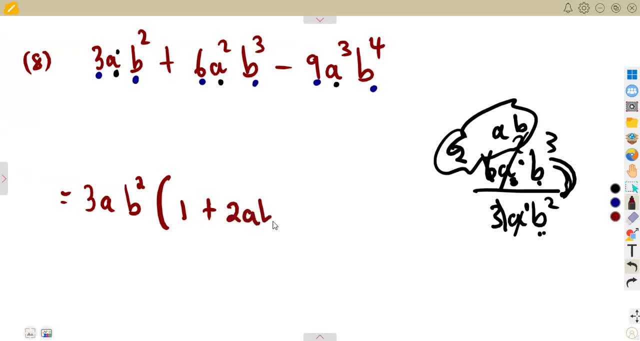 you're gonna have two a b, so this is going to be two a b, all right, minus. you do the same thing on this part of the nine a. so nine divided to three, that's gonna be a three a to the exponent of three divided to a, you're gonna subtract the exponents. if you want to do that, three minus one, that will. 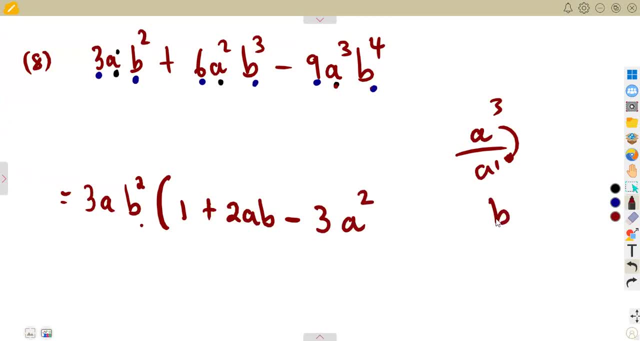 be a squared same thing of b, and the b squared is going to be the exponent of four over b squared. so it's four minus two which is going to be a b squared. so this is what you are going to have and after factoring out the highest common factor, three a, three a b. 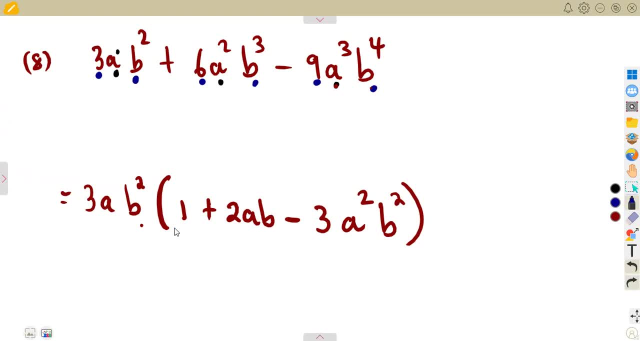 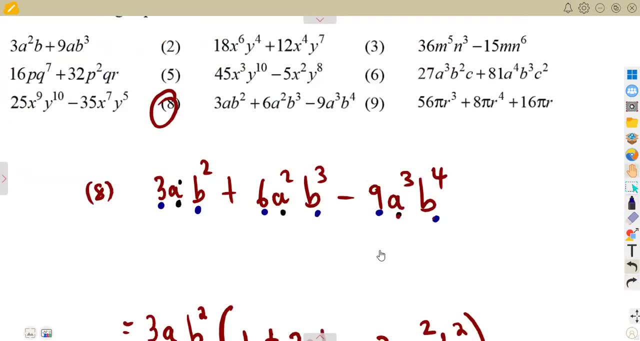 squared. so, in each and every situation that you are going to have, this is how you factorize. uh, whenever there is a highest common factor between the given variables, given terms, whatever terms, number of terms that you are going to have- and the highest common factor between the given.